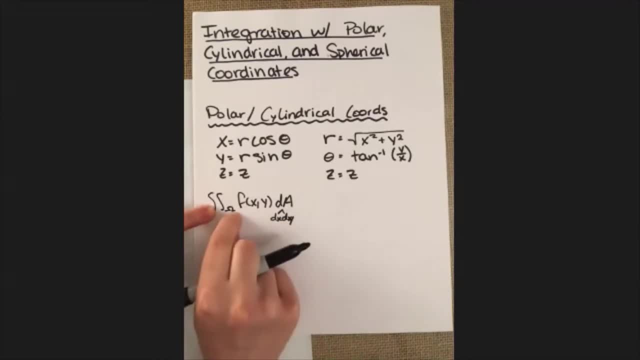 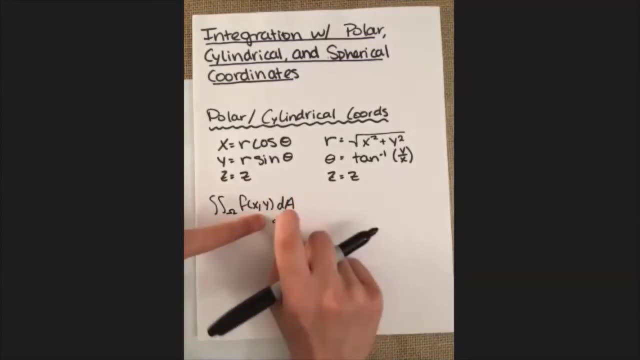 things here that we have to think about converting. We have to think about changing our region over to the polar coordinates, our function over to the polar coordinates and then our final piece here, d a or the d x, d y- over into the polar coordinates as well. So this piece right here is really the 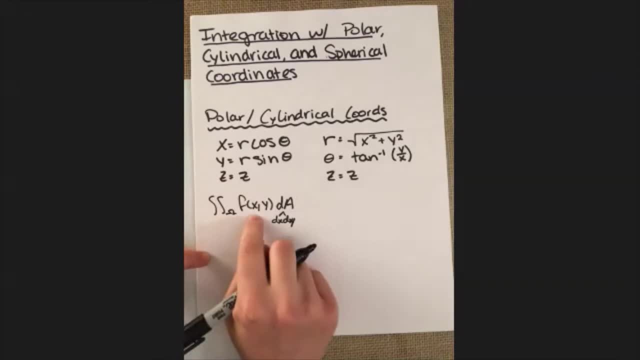 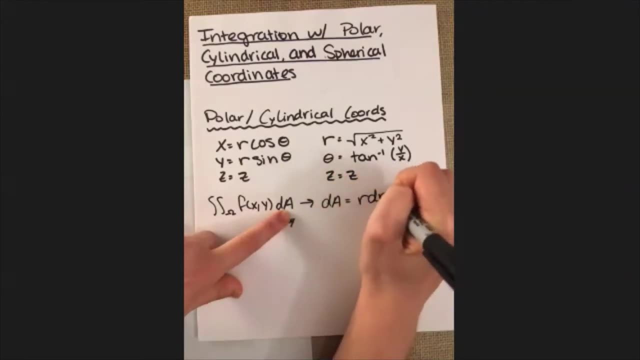 kind of tricky part, because we've seen a lot about how to deal with functions and how to deal with the regions. but this guy right here this turns into r times, dr d theta. because I mean our goal when we're working, when we're trying to move over into the polar or cylindrical coordinates, is to 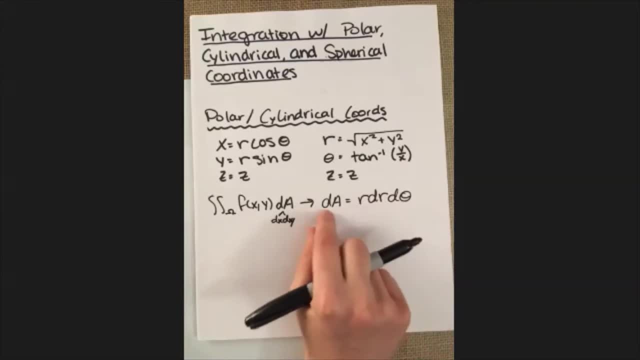 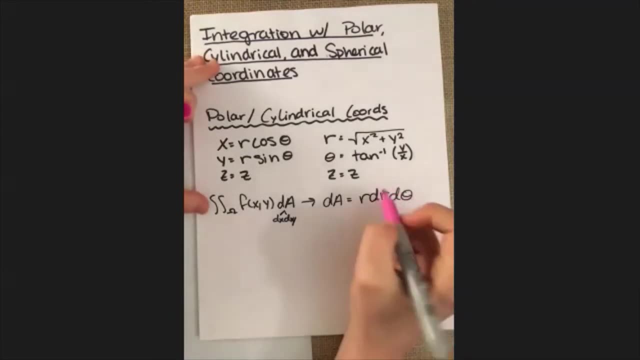 get everything in terms of r and theta. So when we do that for the d a, it just becomes r times, dr d theta. This r here is extremely important. Don't ever forget that The reason that it's there is similar to why maybe some extra pieces might fall off. So if you have a little bit of a problem with 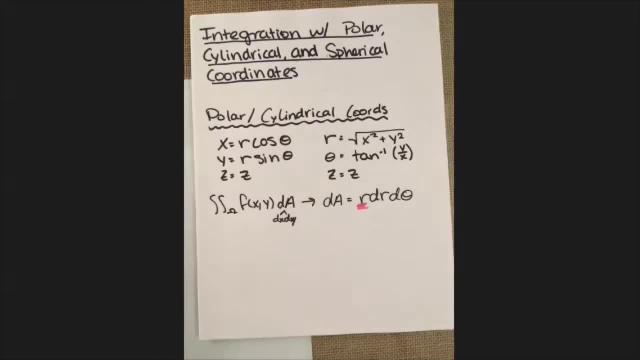 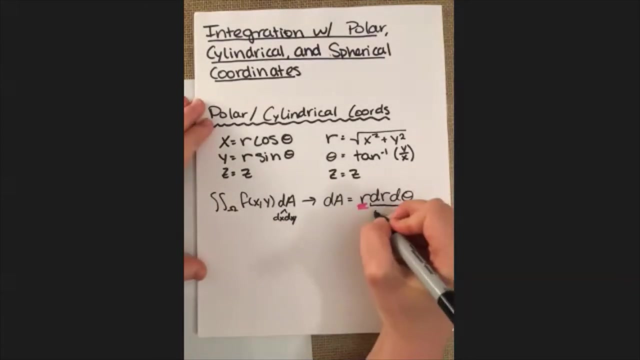 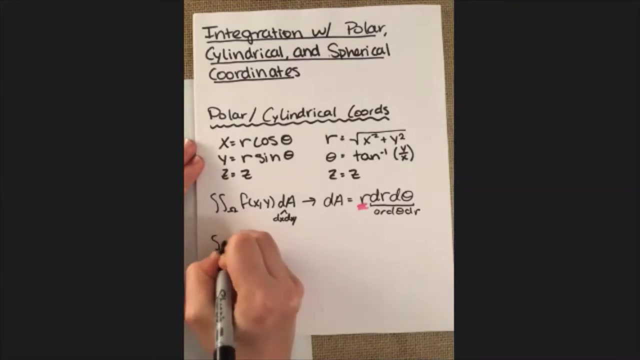 a vector, large for example, and then all the other pieces might pop up in like u-sub for example. it's kind of all related to that, although it's a little bit beyond the scope of this video to go into exactly why that's there. but just don't forget it when we make our swap here And the 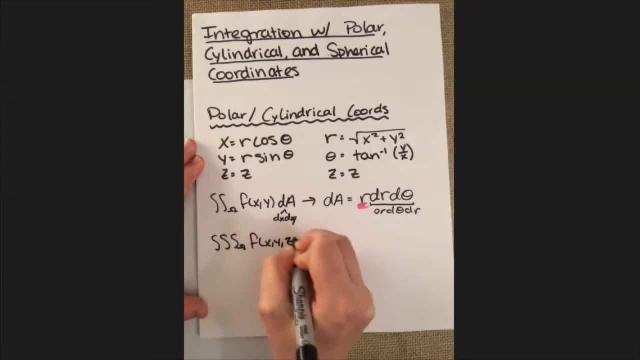 other thing that I want to point out is that these two right here, they can be in really either order, depending on what the problem itself calls for, So this could also be d theta d r instead, And then, instead of DA, we get DV, which is really just the same idea as, like you know, the D, Z, DY, DX or really any other order that we want to put. 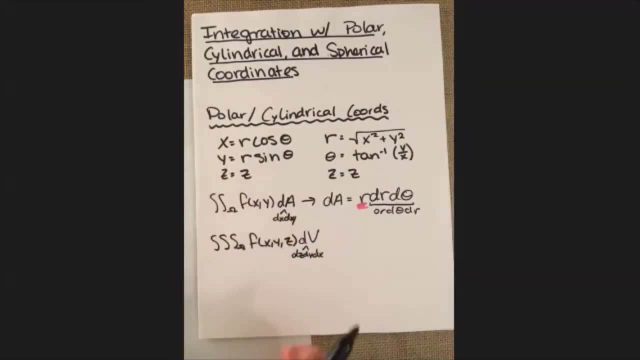 This is just the general expression for all three And again this represents volume, because now we're working in three dimensions. So same idea here: We want to make sure to take care of the region, take care of the function, and then we also have to take care of our little differential type thing here. 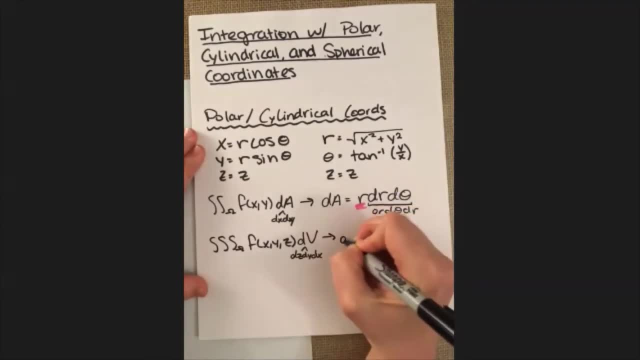 And that is going to be represented with well, R, DR, D, theta, DZ, because really all we're doing here is saying, okay, well, we're still working with this same idea of polar coordinates, but now we're just adding a third component of Z. 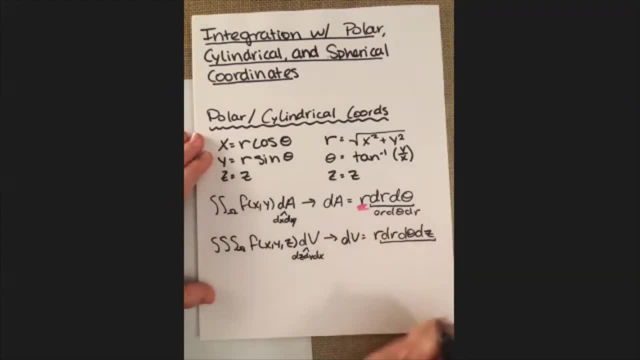 So, again, this can be any order here, depending on what the problem calls for, And then, like I said, we're going to take care of the region. And then, like I said, we're going to take care of the region. 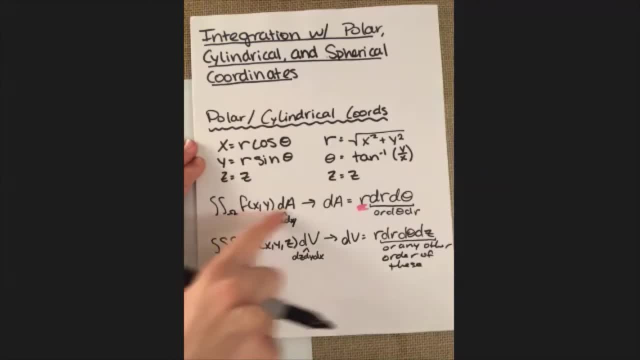 And then, like I said, after you've taken care of your differential, all you got to do is worry about your region and the function. so that's the other two pieces that we have to do. So convert F and your region omega into the polar slash cylindrical expression using your identities. 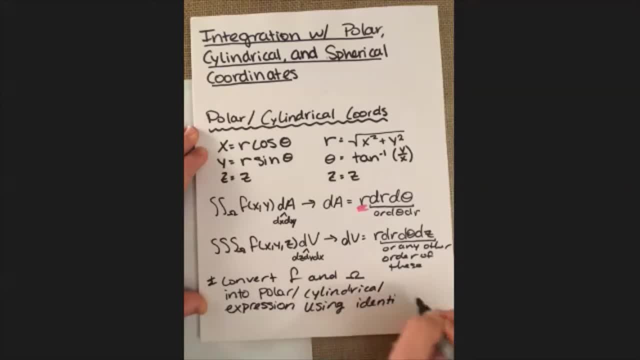 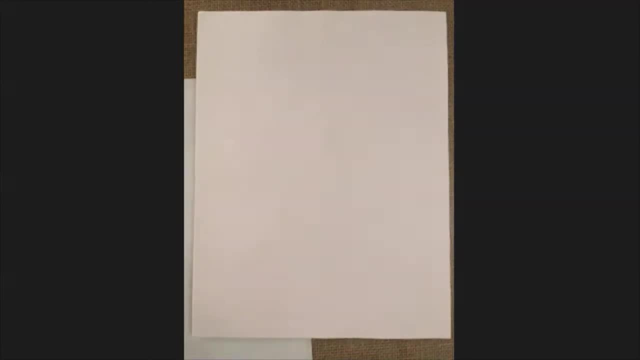 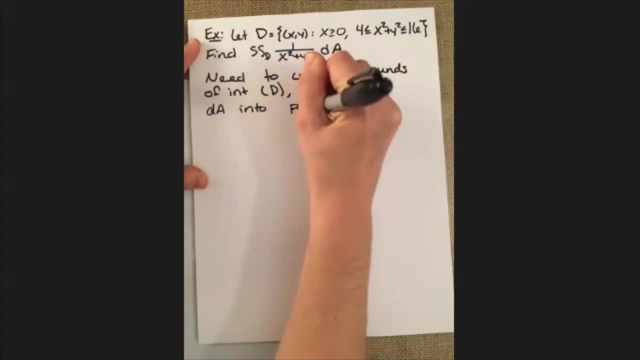 So convert F and your region, omega, into the polar slash cylindrical expression using your identities. And at this point I mean the reason we're working with polar coordinates is because we're not really too concerned about what Z is in this case. So let's go ahead and start with our bounds. 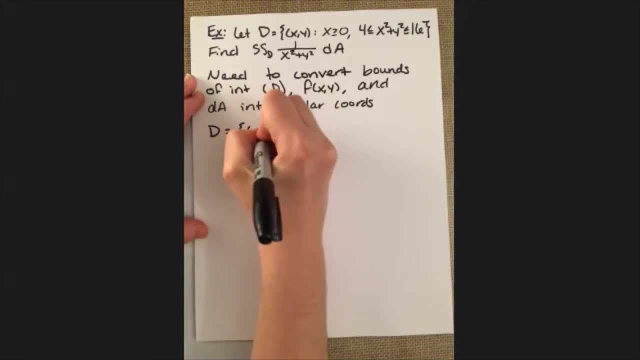 So our goal is going to be to get D to be written as some collection of points- R, theta- And so we just need to find restrictions for R and theta that we can throw into our interval. Let's take a look at what we are. 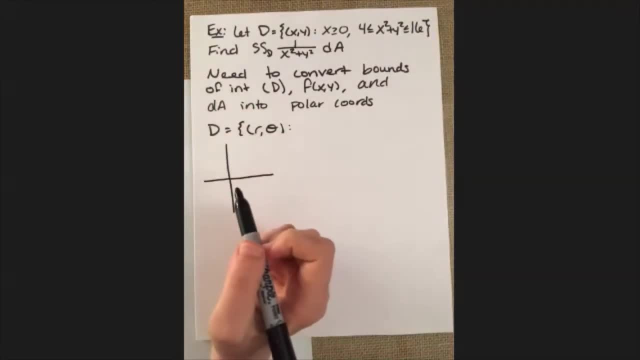 working with here. So we want- it's really kind of like the area between two circles: the circle that has radius two and circle that has radius four. So if this is, we can call it 2,, 2,, 2. And that would be 4.. So we're looking for. 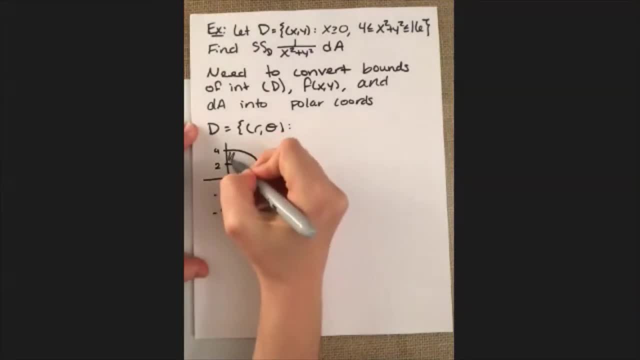 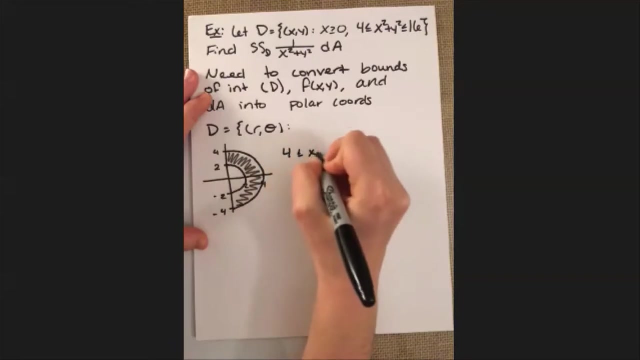 this region right in here, And so we need restrictions for r and we need restrictions for z theta. If we look at this right here, that 4 less than or equal to x squared plus y squared less than or equal to 16.. Remember that r squared is equal to x squared plus y squared, so 4 has to. 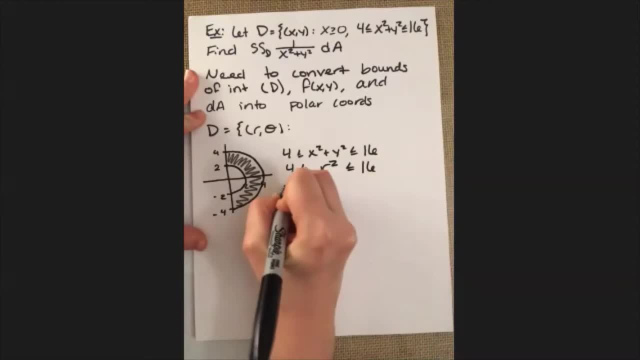 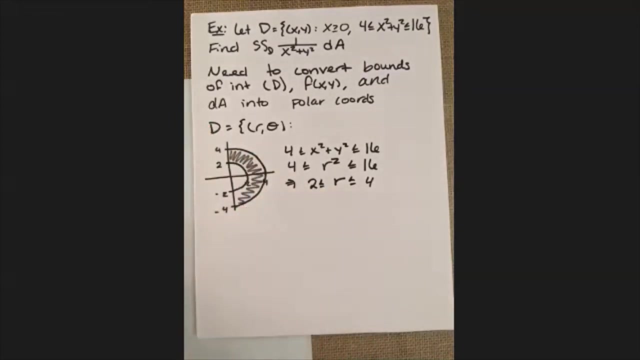 be less than or equal to r squared less than or equal to 16.. So r itself has to be between 2 and 4, which kind of makes sense, because we're looking at the region that is between two circles of radius 2 and has radius 4.. Okay, so the other piece that we have. 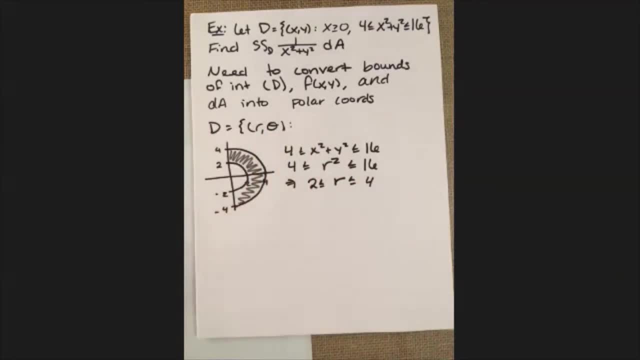 to worry about now is going to be theta, and in worrying about theta we can kind of look at our, I think, here, assign it the ideas from the unit circle. So 0 degrees is along the x-axis, pi over 2 degrees is along the y-axis. You have pi 3, pi over 2 slash. 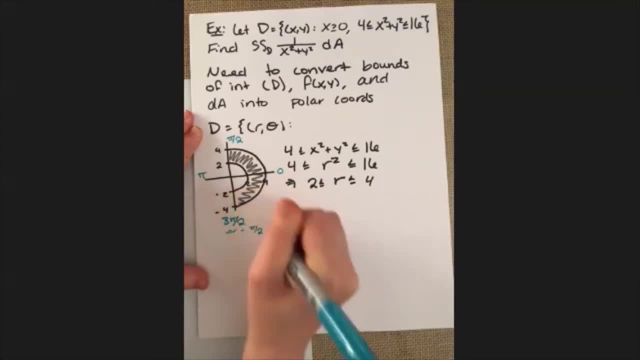 next, theta is along the x-axis, so the radius of theta is along the y-axis and you have to think about theta being equal to pi over 2 degrees or the radius of theta being equal to negative pi over 2, which is really probably what we're going to want here, And we want theta to be able. 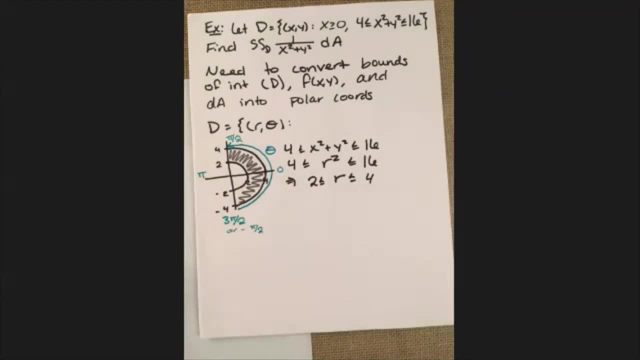 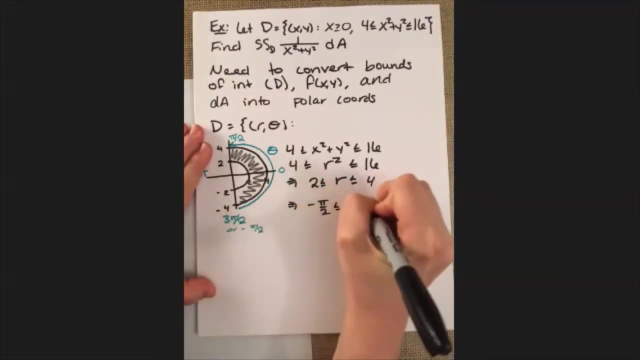 to start all the way down here and go all the way up to pi over 2, so we want it to encompass all of this region here for theta. So that means that our bounds for theta start at negative pi over 2 and end at positive pi over 2.. 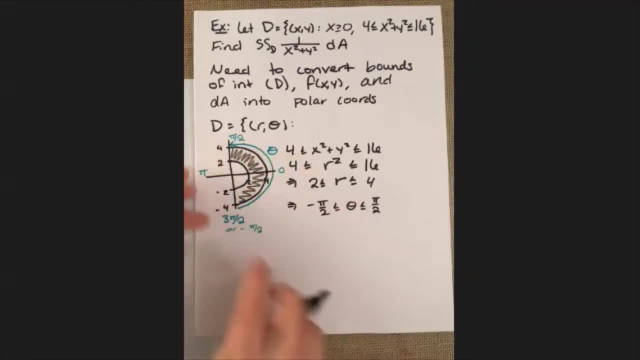 And the reason that we start at negative pi over 2 is because we don't want the root of the original 0 here. so we don't want the root of the original 1 here. so we want only the root of the original because we really just want to make sure that it passes through 0 instead of, like you know, 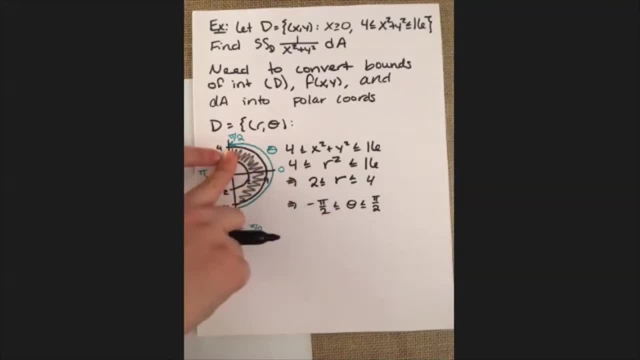 if we start at 3 pi over 2, then we pass through 2 pi and then we pass to. I guess it'd be like 5 pi over 2 or something like that, which really just gets kind of messy. It's a lot cleaner if we. 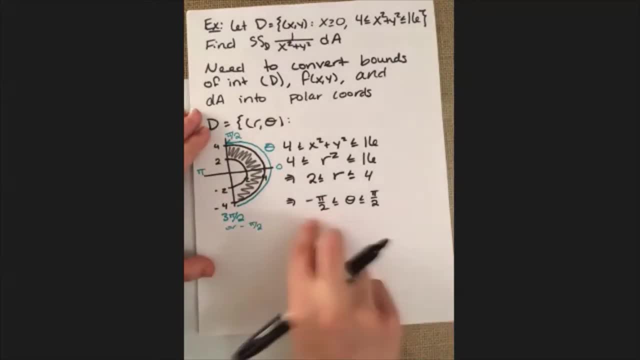 say, start at negative pi over 2, pass through 0, go up to pi over 2.. So these are our bounds for theta and that's what becomes our domain here and that's the information that we'll use to plug into our integrals. So 2 is less than or equal to r, less than or equal to 4, and negative pi over. 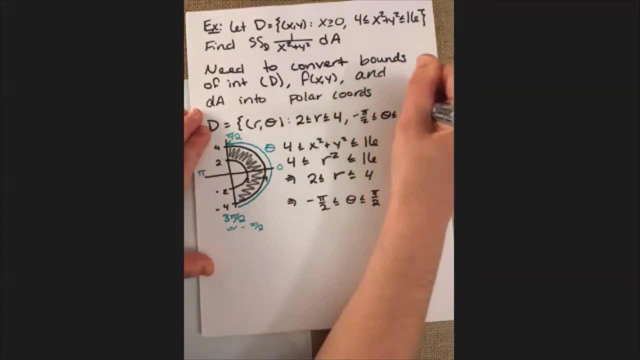 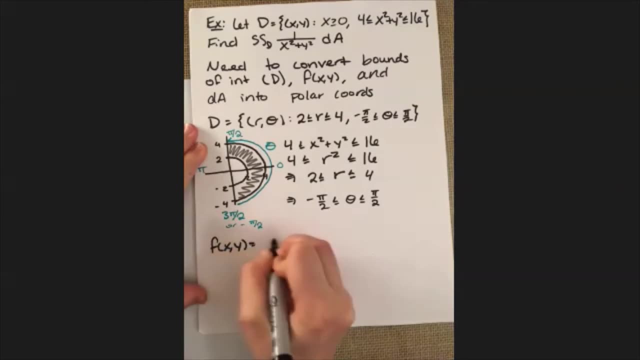 2 is less than or equal to theta, less than or equal to pi over 2.. Okay, and then converting f of x, y is really quite simple here, because this x squared, y squared is just r squared. So that's really all there is to that. And then dA. 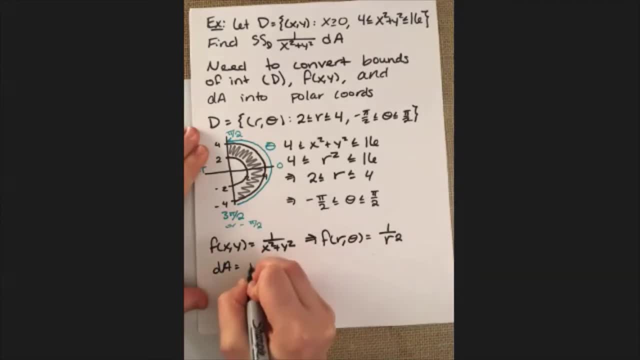 we said was equal to r, dA. This is equal to r, dR, d theta. This is every single time. Do not forget that r there. It's very, very important. So if we want to look at our whole integral, let's put 1 over x squared plus y squared and then dA. This is equal to- and I'm going to fill: 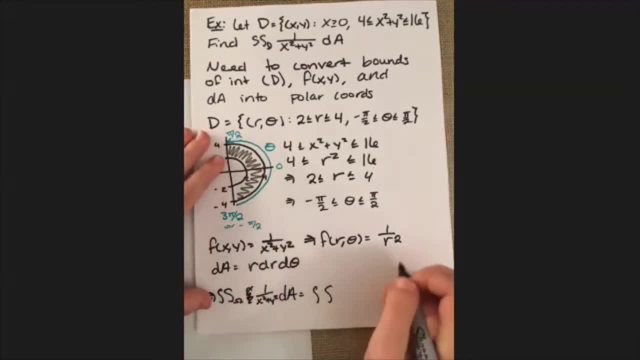 in my bounds after I order my dR d theta- So I have this guy right here- becomes 1 over r squared, The dA becomes r dR d theta, And I just kind of put it in parentheses to denote that this r did not result from converting our 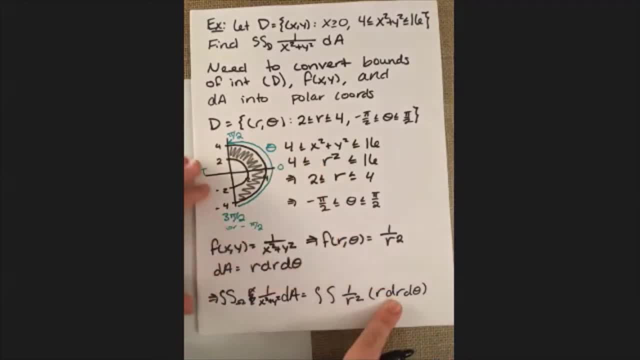 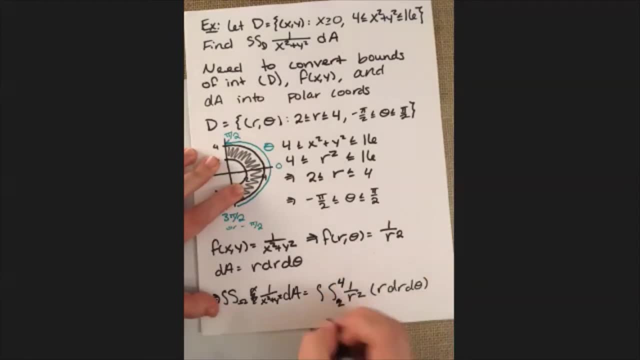 function here, but it'll still get multiplied in. And then, since we're doing r first for our integration, I'm going to put those bounds on the inside, So 2 to 4, and then my bounds for theta would go next at negative: pi over 2,, 2 pi over 2.. So that's pretty much all there is for. 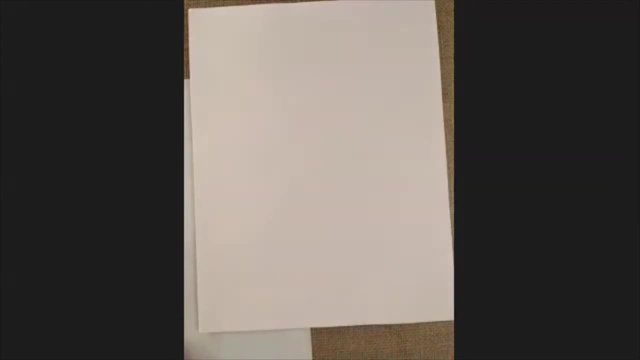 setting up the integral. Let's go ahead and integrate this thing. So we had had negative pi over 2 to pi over 2, integral from 2 to 4, 1 over r, squared r, dR, d theta. So this is equal to the integral from negative pi over 2 to pi over 2, integral from 2 to 4 of 1 over. 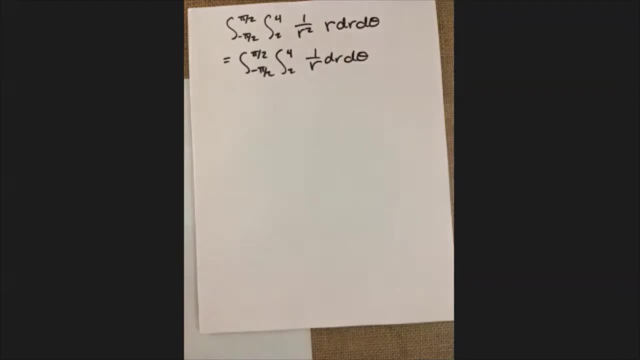 r dR d theta. Well, I mean, this is a fairly simple integral to take. That's just a natural log of r. So we have integral from negative pi over 2 to pi over 2.. So natural log: absolute value of r evaluated from 2 to 4 d theta. 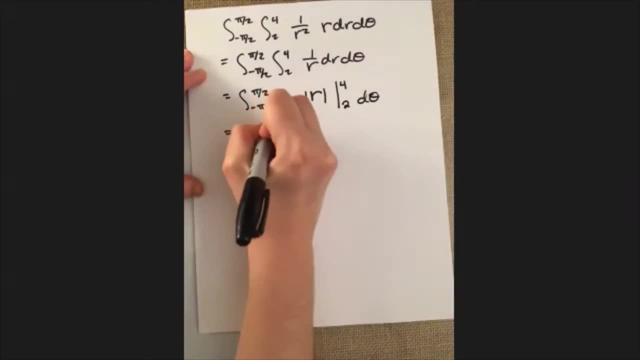 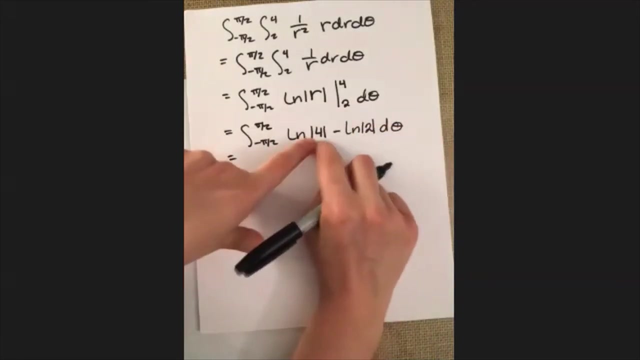 So that's equal to the integral from negative pi over 2 to pi over 2. natural log of 4 minus natural log of 2 d theta. And I can actually kind of simplify this down a little bit farther using log properties. This is the same thing as natural log of 4 divided by 2.. 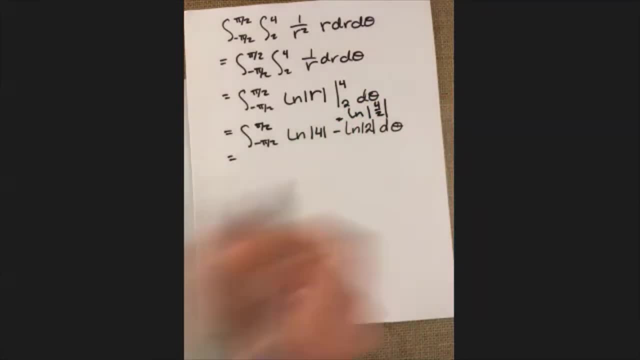 What do I mean by that? 4 over 2.. Like so? So that's just going to give me natural log of 2.. And then we also can integrate with respect to theta here And that's just going to introduce theta and then evaluate from negative pi over 2 to pi over 2.. 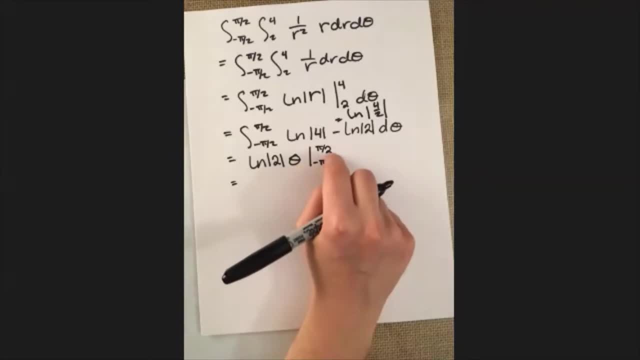 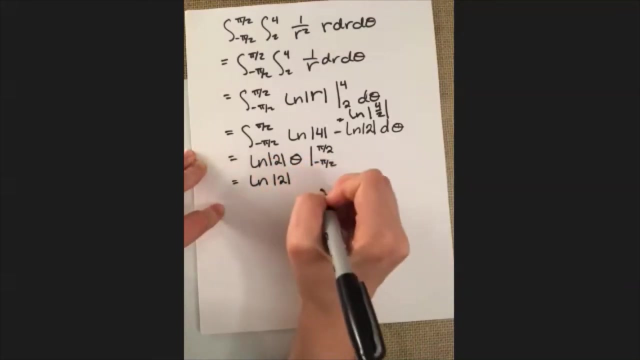 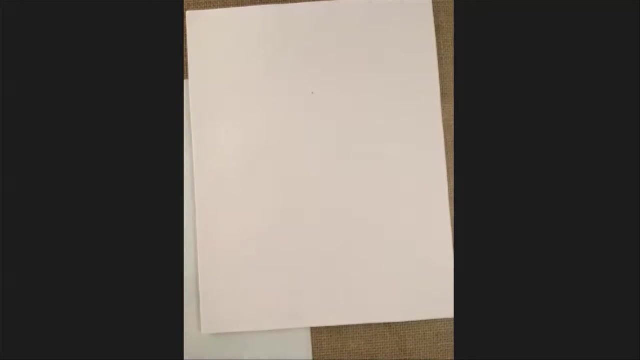 And theta, from negative pi over 2 up to pi over 2, is just going to give me pi And that's really pretty much all there is to that. So that was pretty straightforward. Okay, Let's look at spherical coordinates. So I've already got a sheet set up here with our identities on it. Again, just to remind us of what. 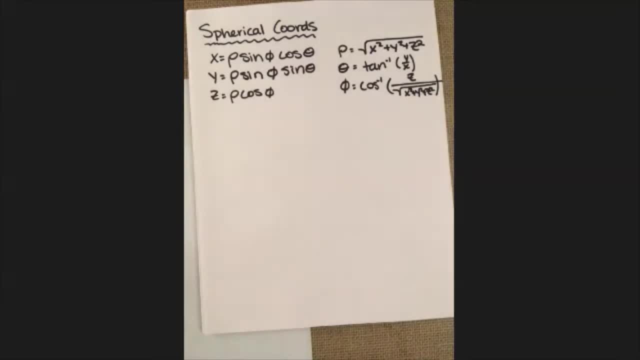 those looked like. So when we're working in spheric coordinates, we're going to have to check the set up. So we're going to need to check the set up and then we're going to need to check the set up coordinates. we're always going to be looking at a triple integral, because spherical coordinates 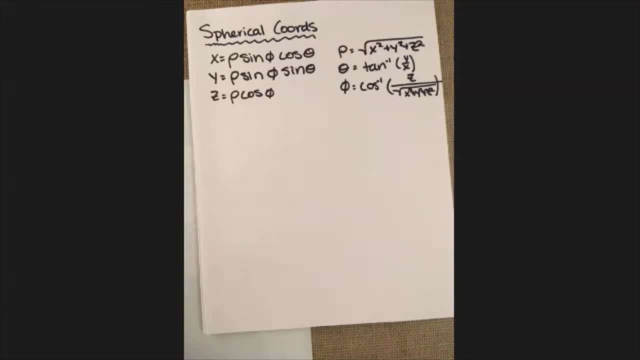 are representative of a three-dimensional space, not like a two-dimensional space, like some cylindrical coordinates could be, or polar coordinates, for example. So we're always going to wind up working with a triple integral. So we have triple integral over omega of some function in terms of x, y and z, and then dv again. Okay, so this is kind of the same setup. 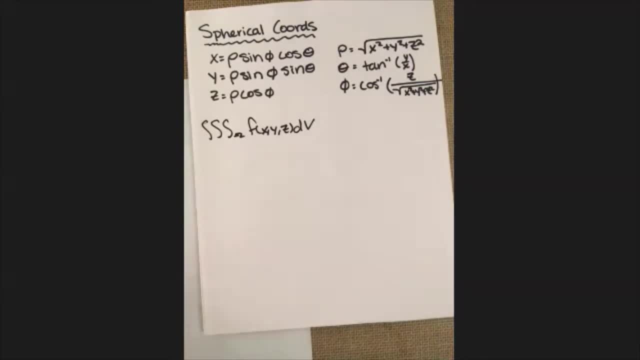 that we started with for the triple integral earlier. dv again is referring to volume, And we still have to deal with converting the bounds, the function and then our differential. So this differential is really the one piece that we haven't talked about yet, just like in the previous. 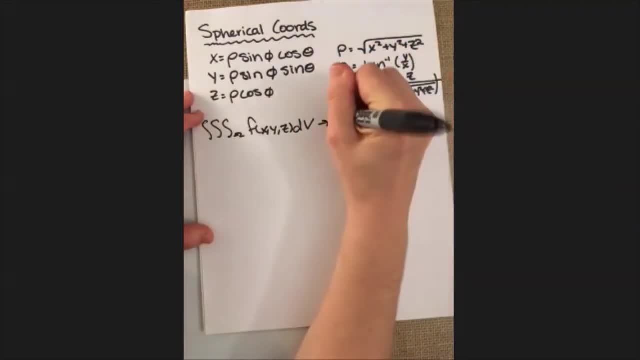 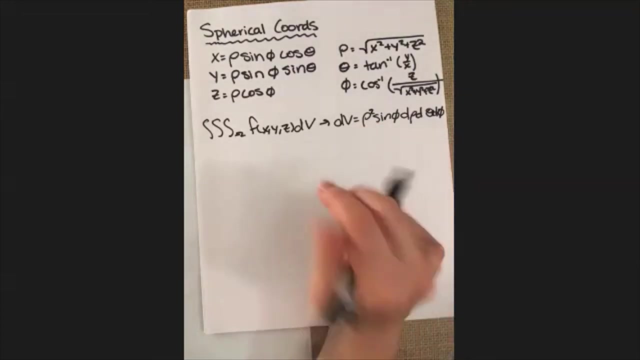 part. So this is going to become rho squared sine of phi, and then d rho, d Theta and then d phi, like so. So it's the same idea here where you wind up with this extra thing that's gotten multiplied in Again. it's part of the same idea of you know, like 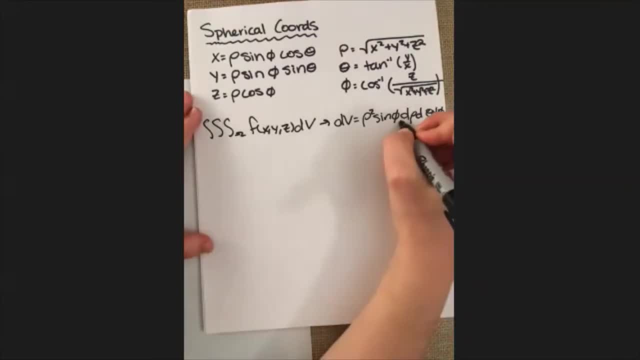 a, u substitution type thing. We are changing the variables And then these guys can be in any order depending on what the problem calls for, And we'll look at a problem in another video, actually a couple of problems in another video where it is actually important. 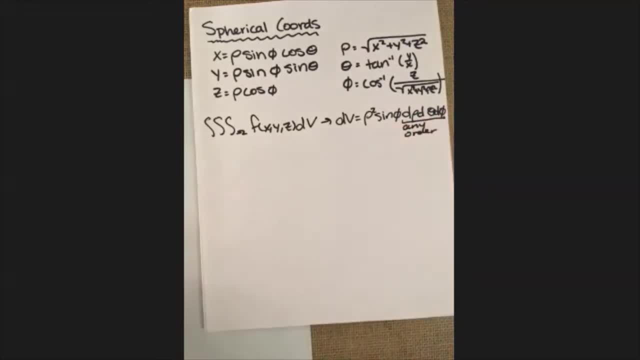 the way that you order these, So you're allowed to rearrange these depending on the needs of the problem. So, oh, make a little note here: Spherical coordinates are always 3D. Okay. so then I mean like, after you've done this piece here, we still have to take care. 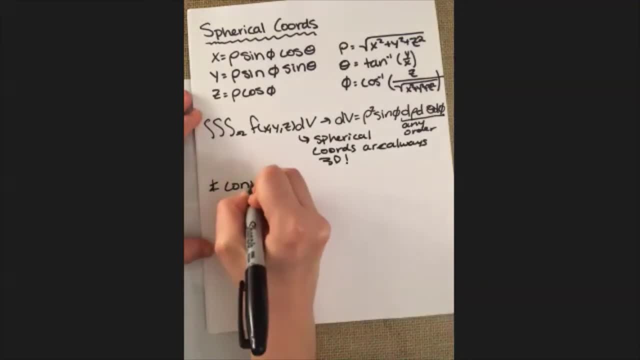 of the boundary and the function. So we also convert f and omega into d, And then we're going to do the same thing over here. So we're going to do the same thing over here, And then we're going to do the same thing over here, And then we're going to do the same. 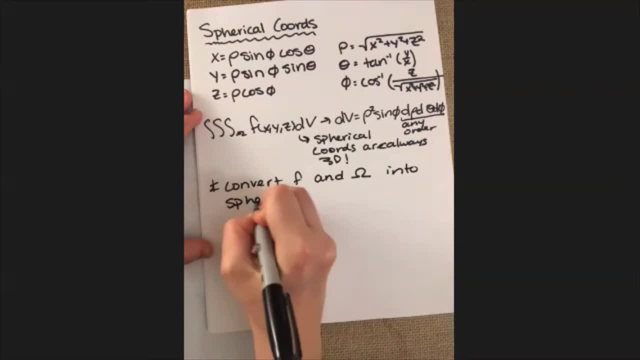 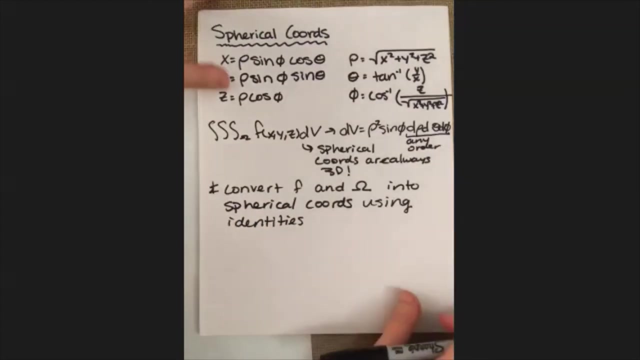 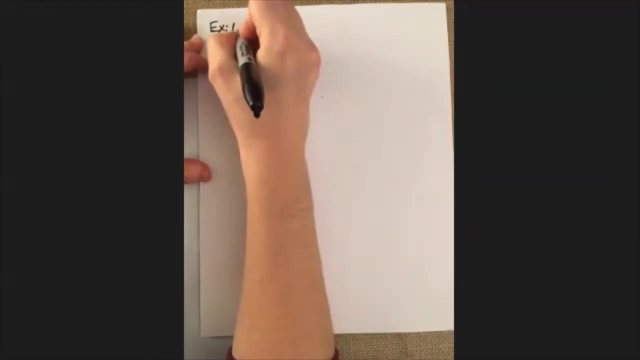 thing over here And, by the way, the portion that's going to disappear in both sides is by using the same thing over here, Up down this part of the equation, So that leads to this Lagrangian. this Lagrangian is going to be minus one half by one half. Or it's going to be minus one half over� plus 1, butclipse is always the same n, because it's less than or equal to a, tends to be, or less than or equal to a, So it's its full value, Right? So if we just connect back to the function, we know that t is a fixed. value. right here, We know that t is great. The mean constant- All right, Another question, So we're going to use these terms to solve right now. Butkolà, here's our last one. We're done with the quiz, So let's go ahead and do the next one. This one about course, order 포인ating. 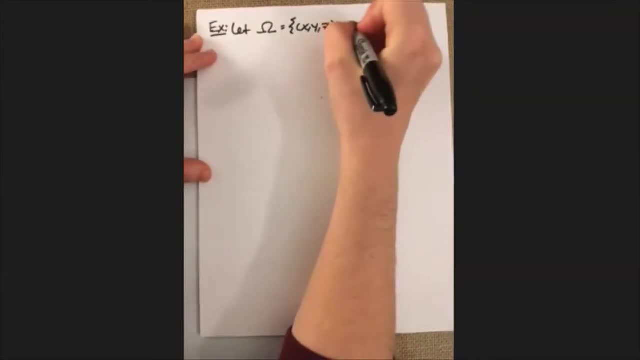 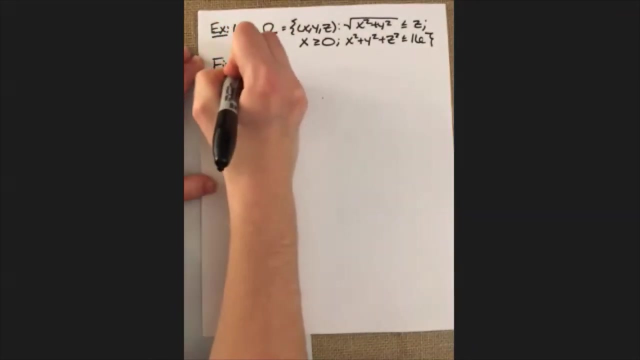 z, such that the square root of x squared plus y squared is less than or equal to z. x is greater than or equal to zero. and we also have that x squared plus y squared plus z squared is less than or equal to 16.. And we are going to find the triple integral over omega. 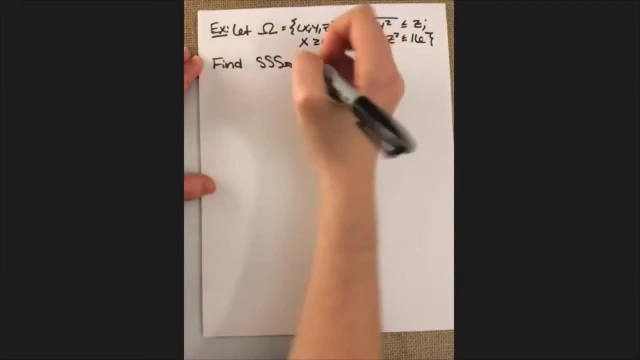 of x times dv, or well, not times dv but xdv. So the way to approach this, since we've kind of got some a boundary here that looks like a sphere, it would really kind of might be a good idea to approach this using spherical coordinates. but, and actually, if we kind of remember back to, 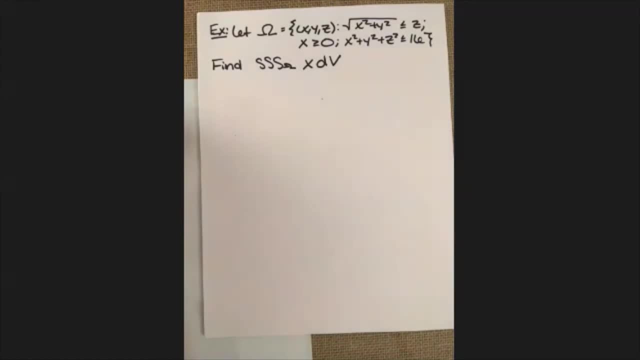 our video earlier, our first video on the cylindrical and spherical coordinates. this is really quite a similar setup. The only thing is that we've just kind of chopped our reading region in half by requiring x to be greater than zero. So let's take a look at what our 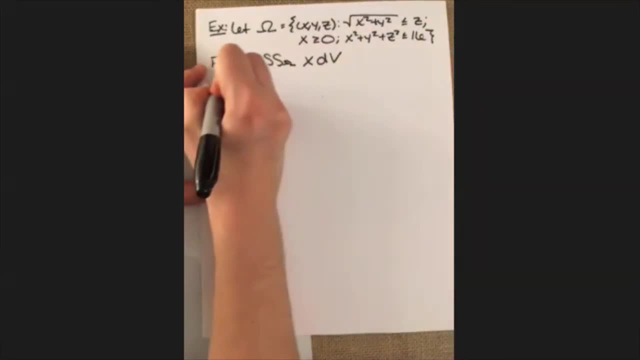 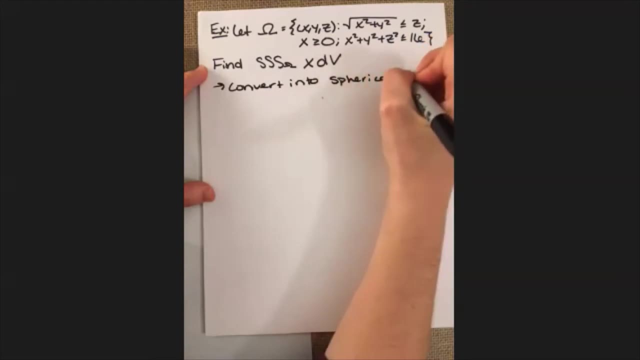 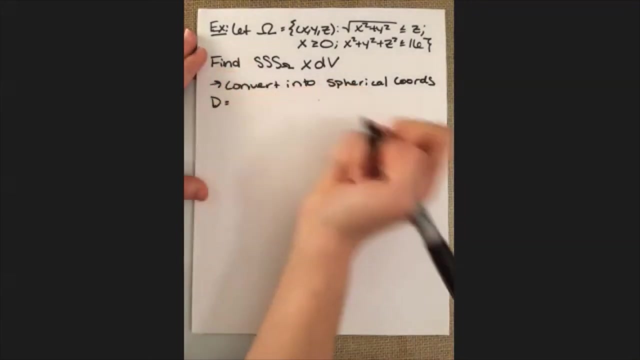 space looks like, but this will wind up being spherical coordinates. So our goal is going to be to take our domain and write it as rho theta phi, and then we've got to come up with a structure. So we're going to take our domain and write it as rho theta phi, and then we've got to come up with a structure. 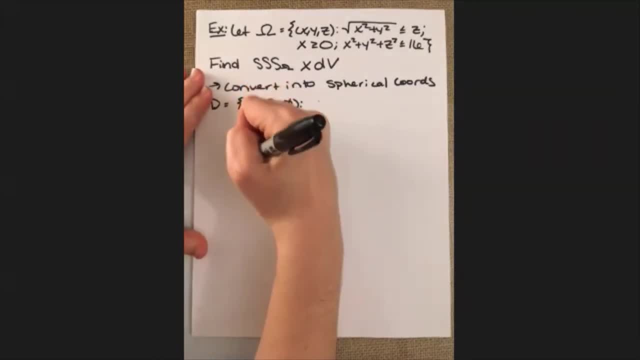 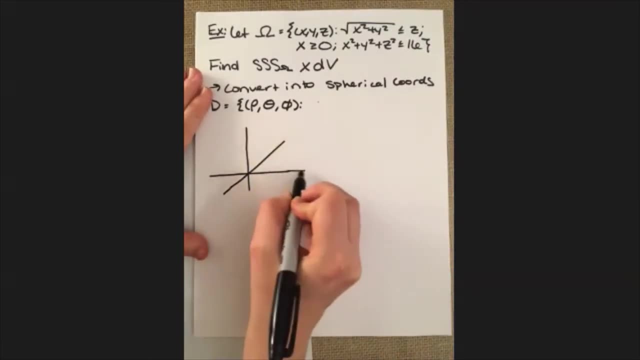 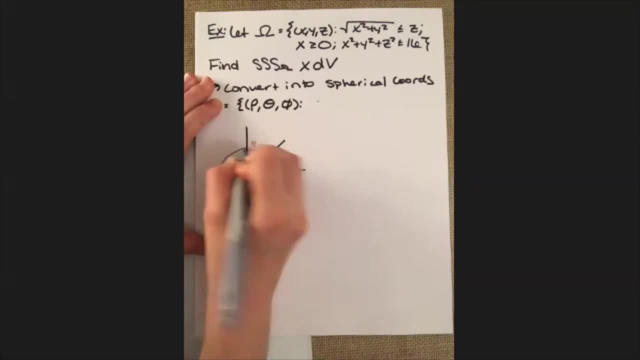 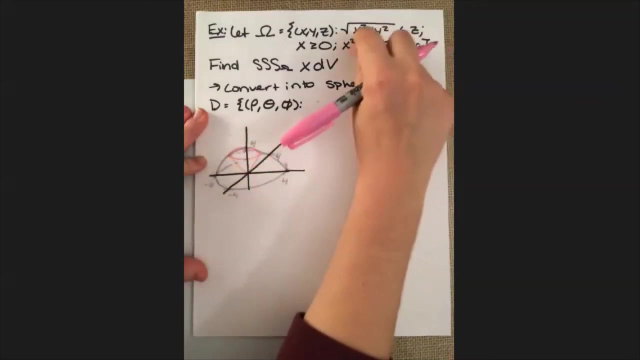 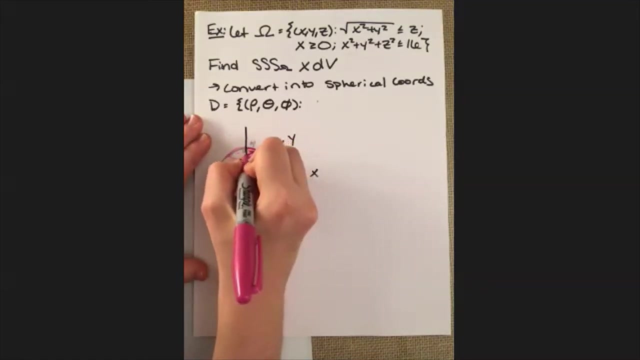 we're going to take our domain and write it as rho theta phi, and then we're going to take our domain and write it as rho theta phi. and we're going to take our domain and write it as rho theta phi, and then we're going to take our domain and write it as rho theta phi. 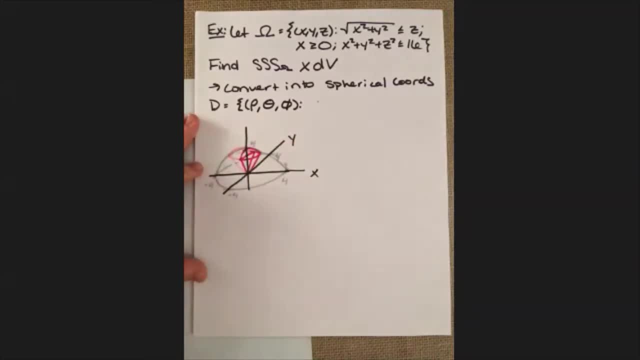 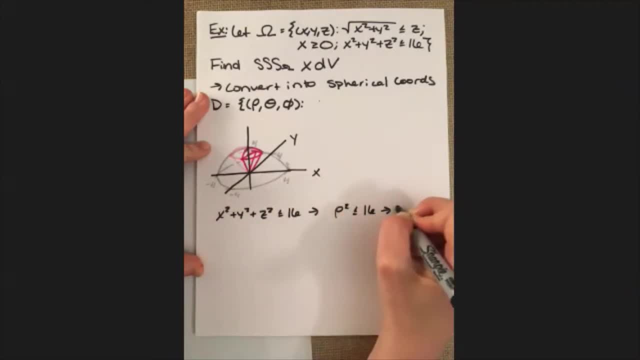 so rho squared has to be less than or equal to 16, which means that rho has to be between 0 and 4.. And that kind of makes sense because if we look at what we want rho to be, we want it to kind of start down here at the base and then go up here and touch the top of that. 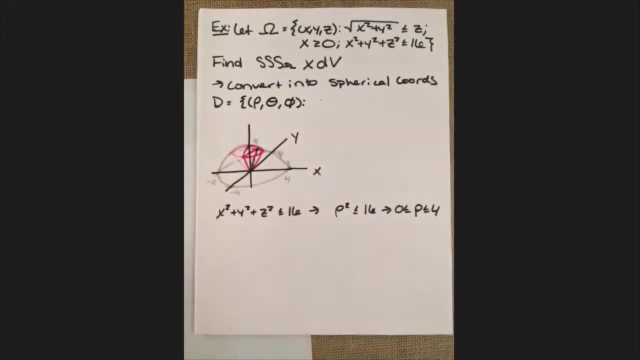 sphere, which means that it has to have, well, the radius 4 of the sphere. Now looking at theta, theta is also going to be fairly straightforward, because that's what tells us how much it sweeps out in the x and the y axis, or x and y plane, and we only want the part that. 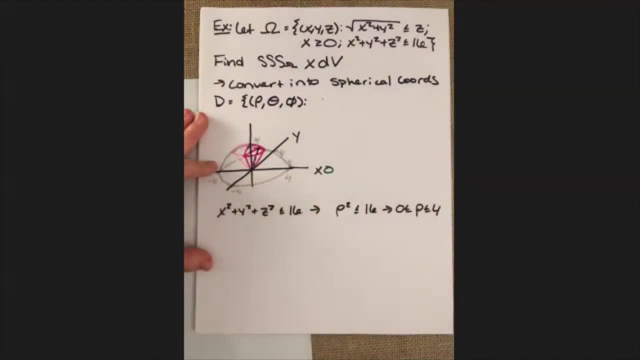 goes from again, if this is 0 pointing in the positive x direction, and then pi over 2 in the positive y direction, pi and then 3, pi over 2 over here in the negative y direction, We want it to start down here and be able to come up and around this way, only taking half of our xy plane. 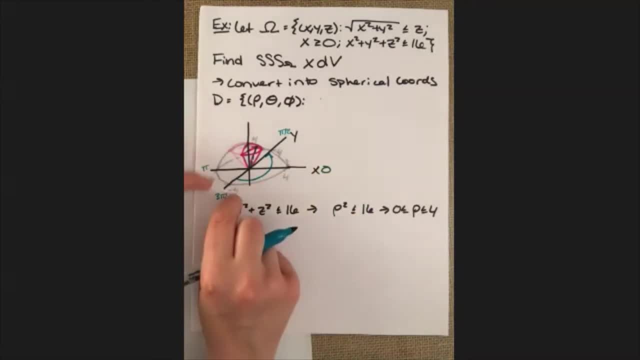 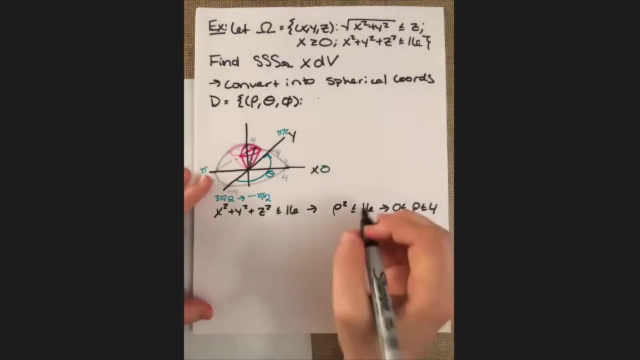 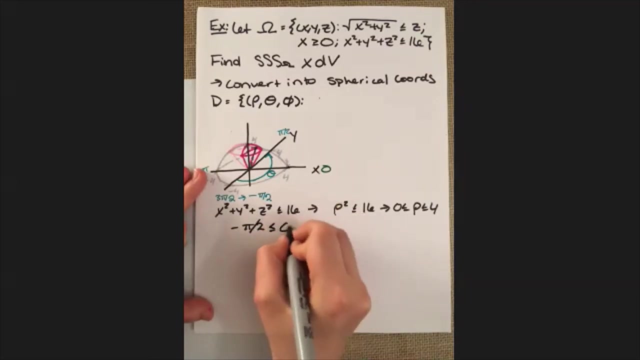 but we always want it to be the half that x is positive in, and that is going from well, negative pi over 2 up to pi over 2.. And that's for theta. So we know that negative pi over 2 is less than or equal to theta, less than or equal to pi over 2.. 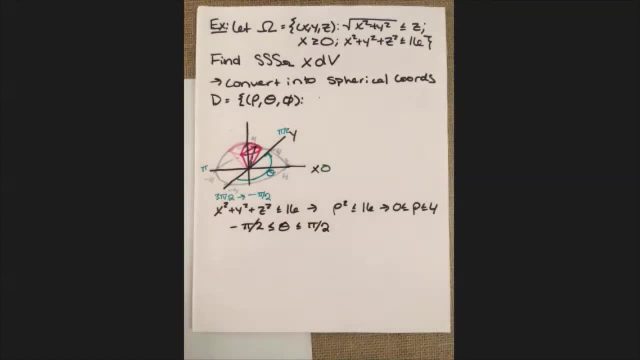 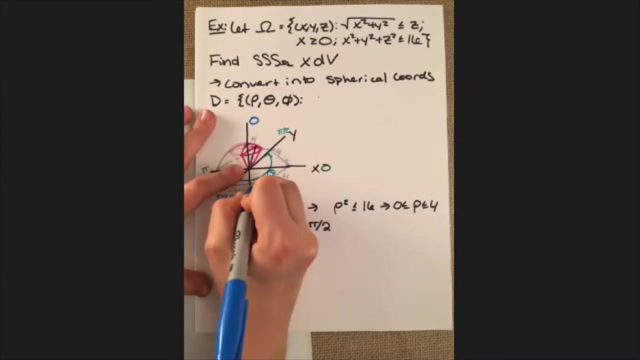 And we also determined in our previous video that phi, which is what goes from along our z-axis, here it starts at 0 and is able to go all the way down to pi. if we go down to the negative z-axis, here, We want it to start at 0, and that's what we're trying to get out of the equation here. 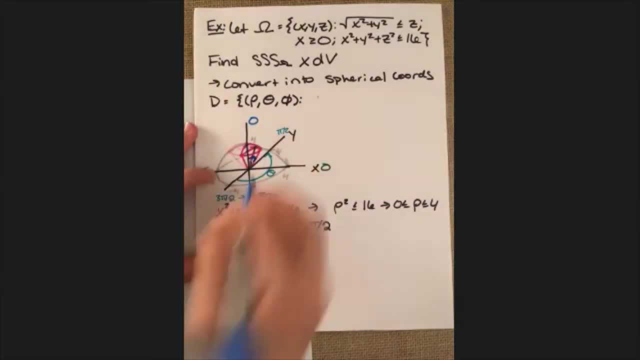 So we know that negative pi over 2 is less than or equal to pi over 2, and that's what we're going to do here with this recall from our negative pi over 2, and we know that negative start at 0 and be able to go out to this line right here, which is really just pi over 4.. 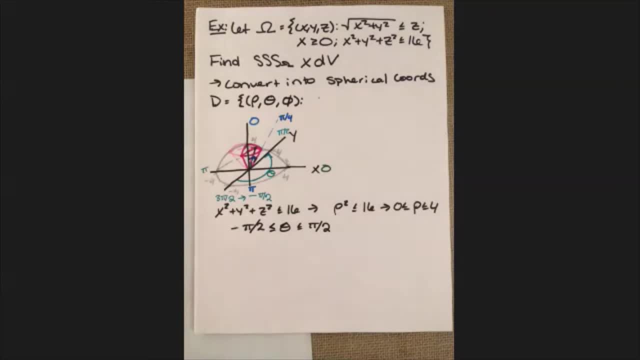 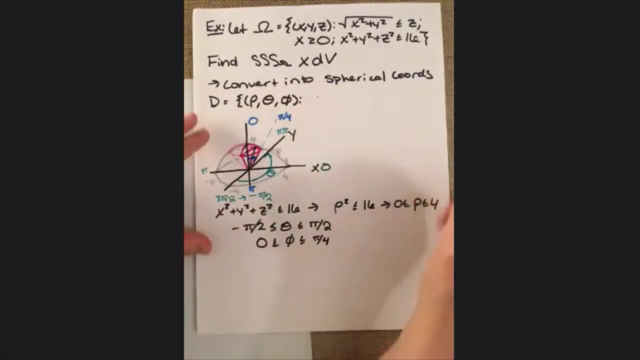 So it's allowed to swing down pi over 4 degrees or radians. So it starts at 0,. can only go halfway down to the xy plane. so that's pi over 4, just like so. Okay, so that's what we're going to use to describe our domain here. 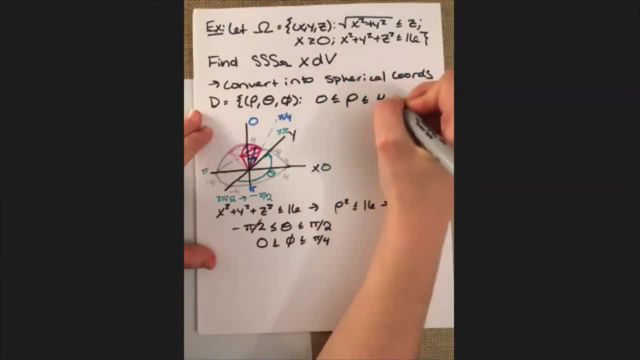 Rho is between 0 and 4.. Theta is between negative pi over 2 and positive pi over 2.. And then phi is between 0 and pi over 4.. So these are going to form our bounds of integration here And now. we still have to convert the inside and our dv. 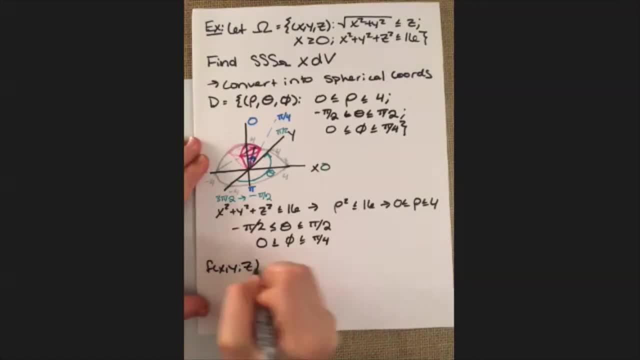 So f of xy z is equal to x, which means that when we take f and write it in terms of rho, theta and phi, we're going to get- if we go back to our identities- x is equal to rho sine, phi, cosine theta. 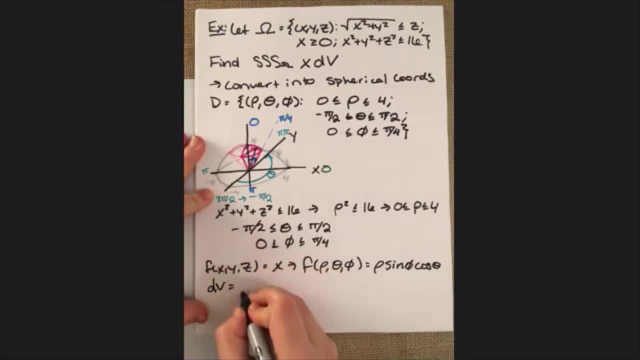 And then we said that dv is equal to rho squared sine phi d rho d theta d phi. So if we want to rewrite this completely, triple integral over omega x, dv is equal to well, we still have a triple integral. 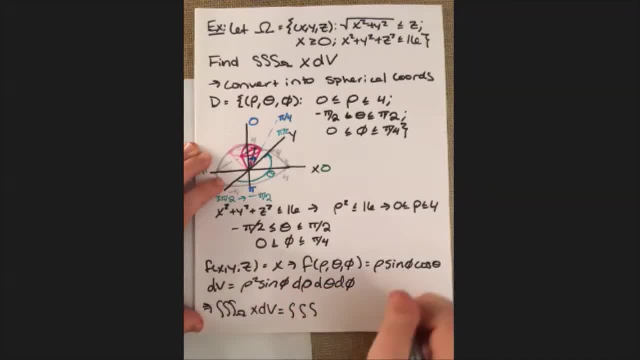 And then we have x becomes rho sine phi phi, cosine, theta phi, squared sine of oh, no, okay. And then we have d rho d theta d phi. This is all attached to the end of this integral. I just ran out of space there. 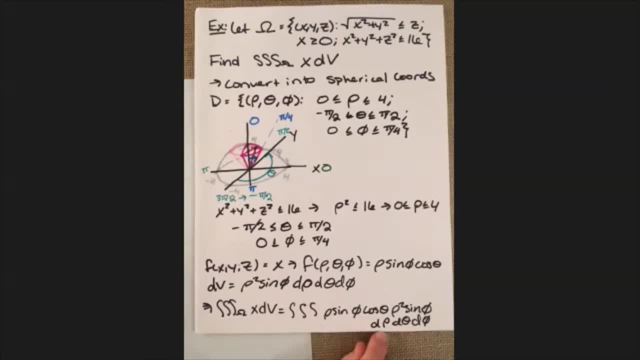 And then I still have to define my bounds of integration according to this order right here. So we're starting with rho, which goes from 0 to 4.. d theta, which is going to go from negative pi over 2 to pi over 2.. 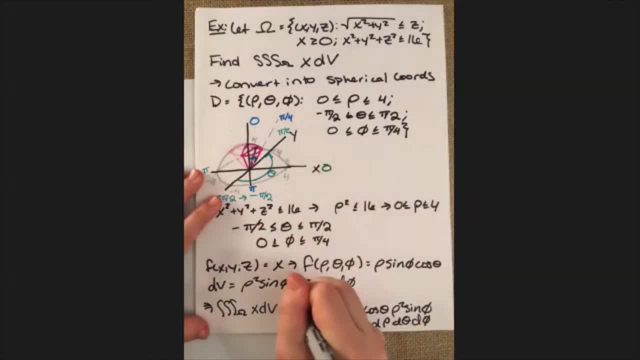 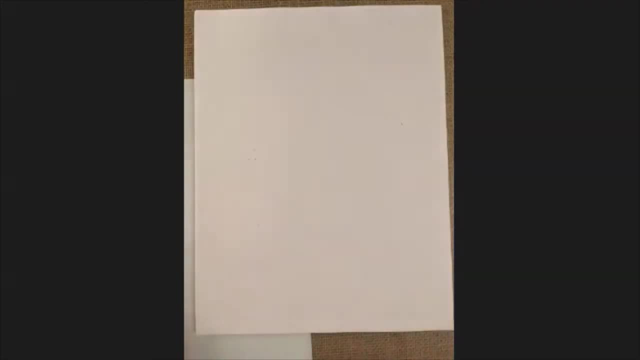 And then phi is between 0 and pi over 4.. And that's pretty much all there is to setting up that integral. Let's go ahead and integrate it. So we had integral from 0 to pi over 4, integral from negative pi over 2 to pi over 2,. 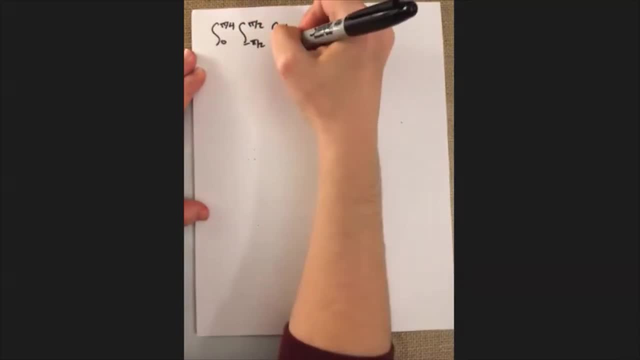 and integral from 0 to 4, rho sine phi, cosine theta- And I'm going to run out of space- again- Rho sine of phi, And then d rho d theta, d phi Again. ideally, all this would be on the same line. 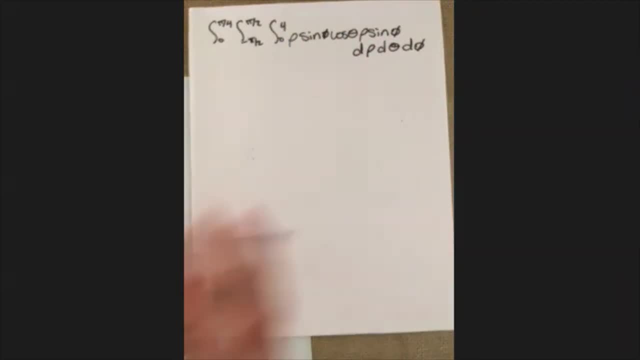 but apparently I just didn't plan ahead well enough, So but I mean, like I can compress this down a little bit, This is the integral from 0 to pi over 4, integral from negative pi over 2 to pi over 2,. 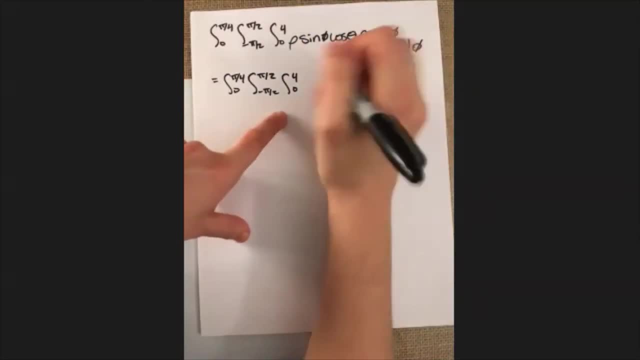 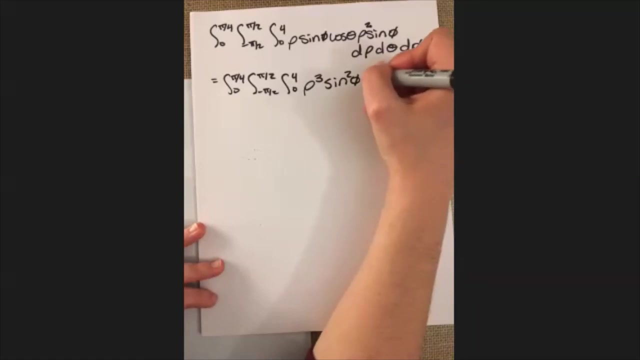 integral from 0 to 4 of it'll be rho. oh no, Yeah, rho squared. So we'll have rho cubed sine squared, phi Cosine, theta And then d rho, d theta, d phi. So then I can go ahead, since everything here is just a product of different pieces here. 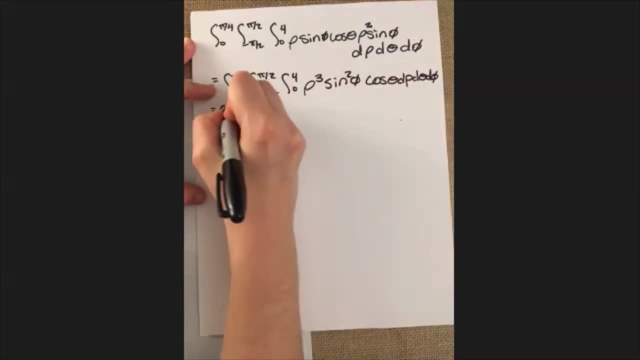 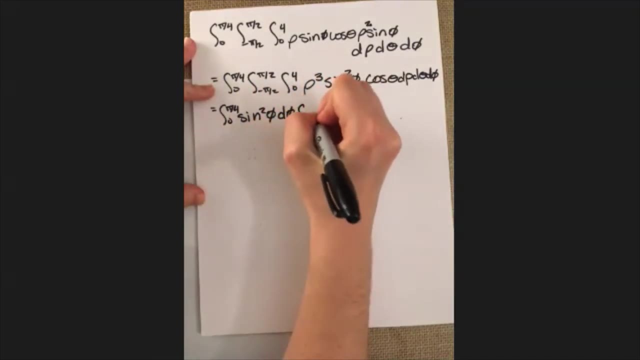 I can split it up into you know two product of integrals. So I get 0 to pi over 4 of my phi function, And then integral from negative pi over 2 to pi over 2 of my theta function, And then integral from 0 to 4 of rho cubed d rho. 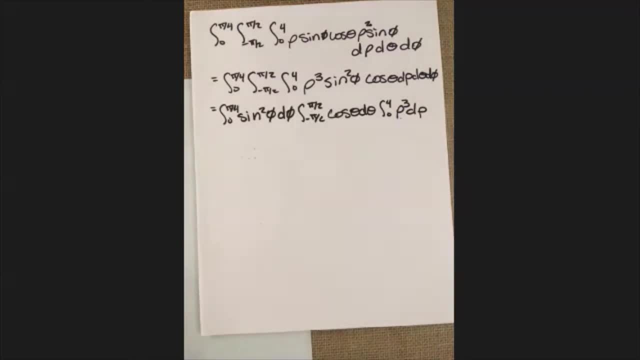 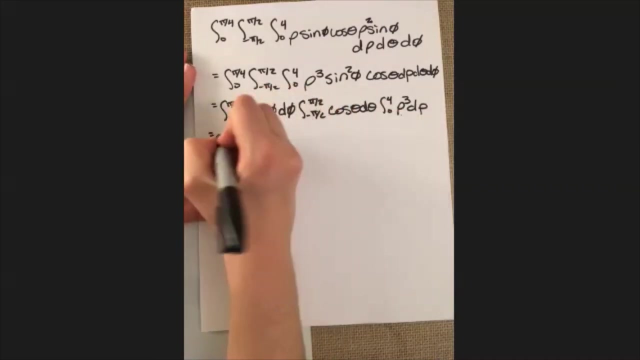 Okay, So now at this point I can integrate each one of these pieces individually. this one right here. I recommend using a power reduction formula for sine squared. There's also one for cosine squared that's quite similar: 0 to pi over 4 of it's one half. 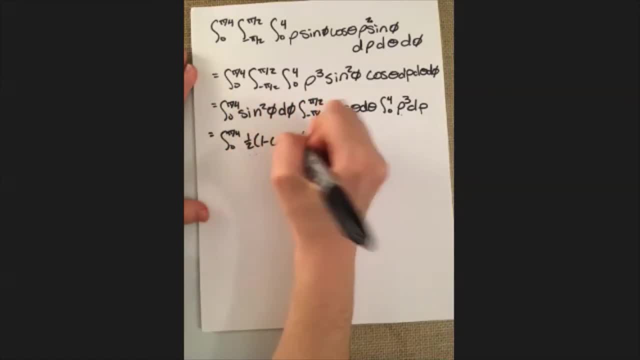 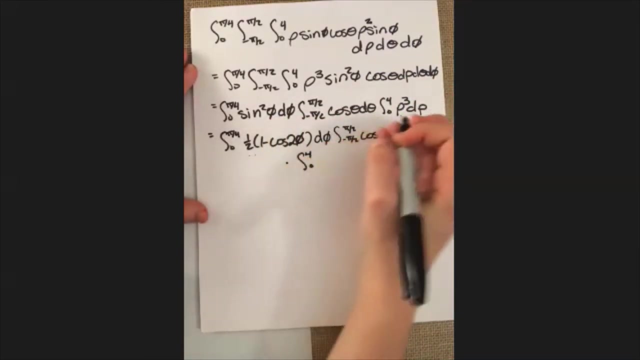 1 minus cosine 2, phi is what we get there. d phi integral from negative pi over 2 to pi over 2 of cosine theta, d theta. And then this is times, not plus integral from 0 to 4: rho, cubed d rho. 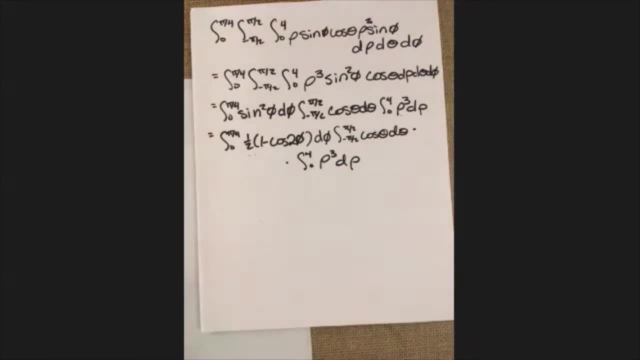 Now, each one of these you just kind of integrate the way that you normally would And from this we're going to get 1 half theta minus 1 fourth sine of 2, oops, that shouldn't be a theta. 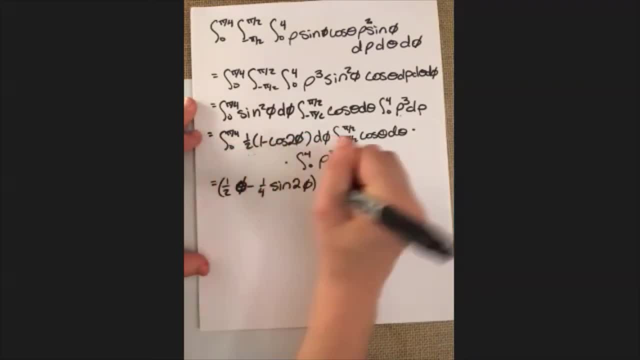 that should be a phi 2 phi. And then this is times this integral. right here I'm going to get sine of theta evaluated from. ah. got to evaluate this one: 0 to pi over 4.. This is evaluated from negative pi over 2 to pi over 2.. 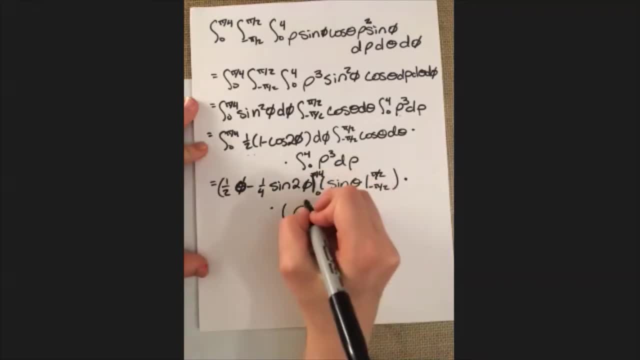 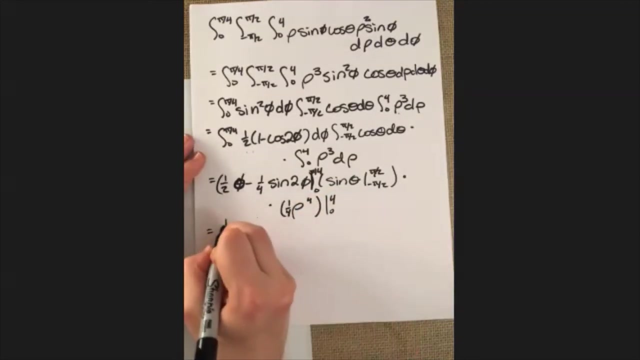 And then this is times, once again: rho 1, fourth rho to the fourth, 0 to 4.. So out of this what we're going to get just plugging everything in, so 1 half times pi over 4 minus 1 fourth sine of. 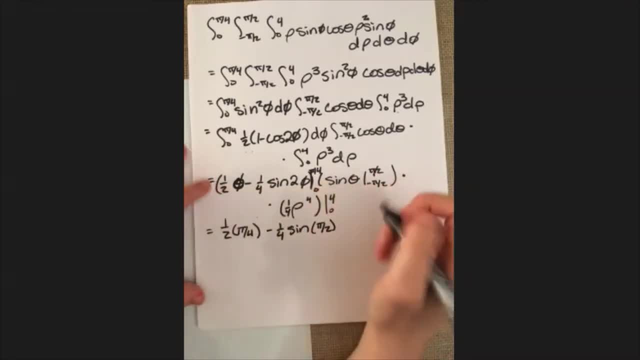 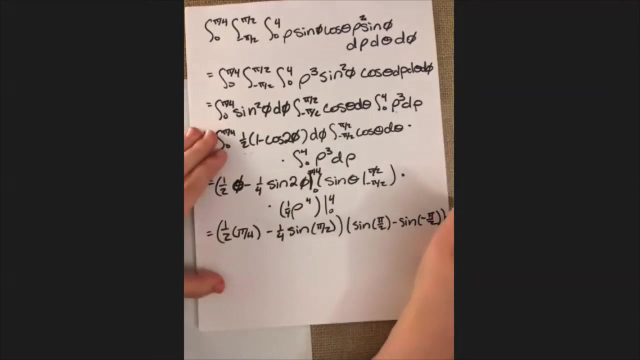 it'll be pi over 2.. And then this next piece will be 0, so I'm just going to leave that off. times sine evaluated from pi over 2, minus sine of of negative pi over 2, and then times 1, fourth rho to the fourth. 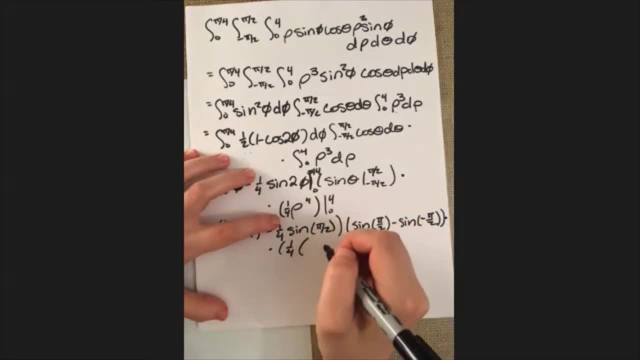 and 4 raised to the fourth, power is going to be 256.. All right, so from this I'm going to get pi over 8 minus. this is 1 fourth times this right here it's just going to wind up being 2,. 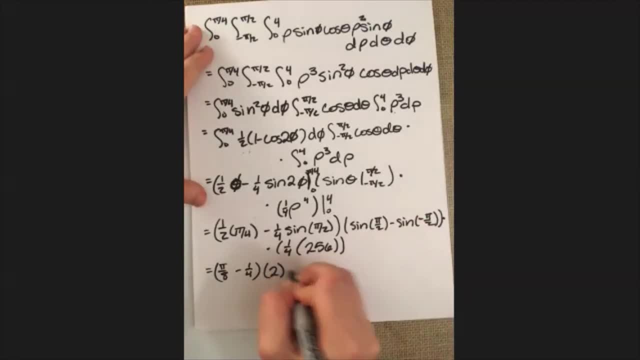 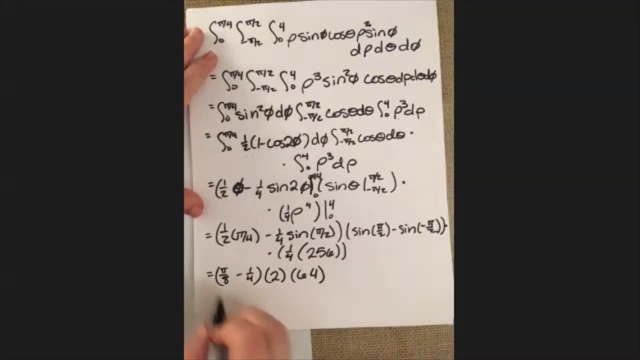 because we have a 1 minus negative 1,, so 2, and then times 1, fourth times 64, that's going to give me, or 256, that gives me 64. So 128 divided by 8 should be.